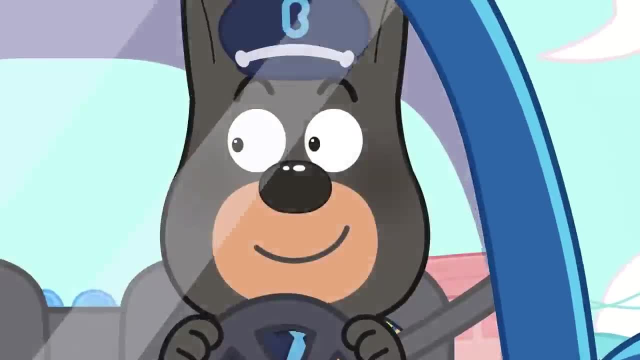 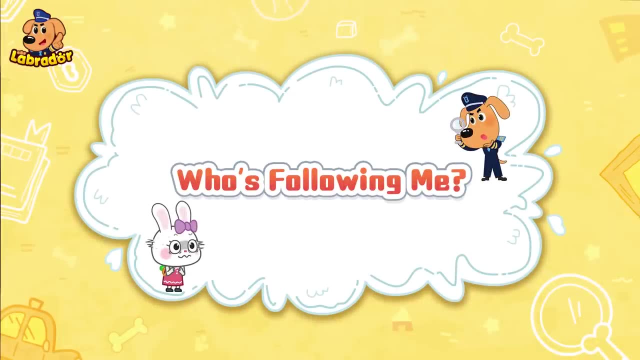 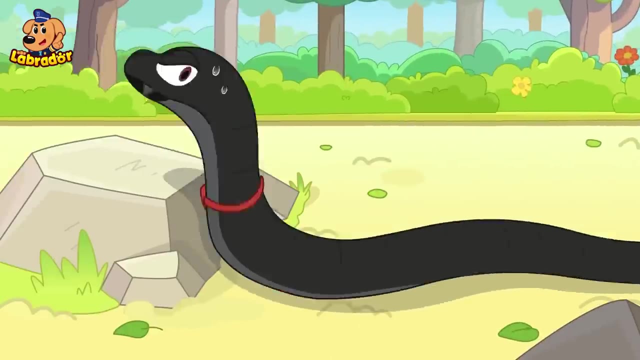 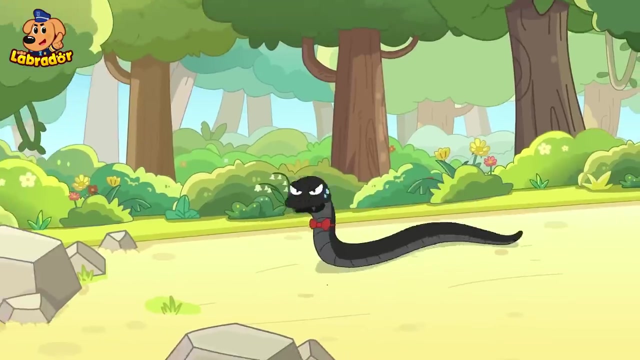 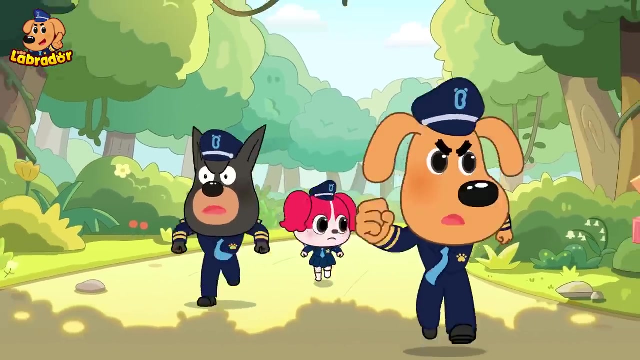 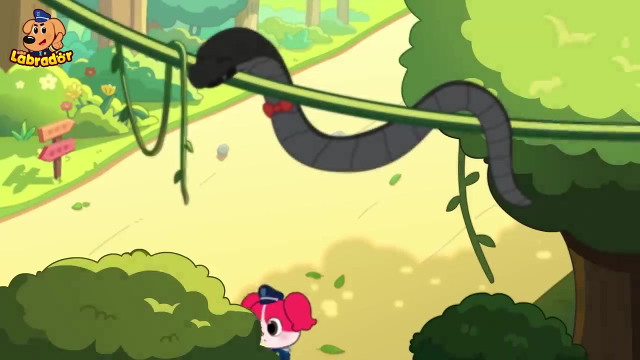 Go, go, go go. Let's go. Sherry Labrador, Who's following me? Stop right there. Oh no, Black Mamba got away again. We need to catch him before he harms other kids. Phew, Finally got away from the police. 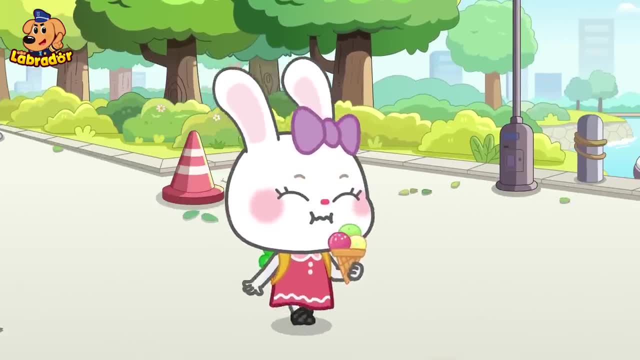 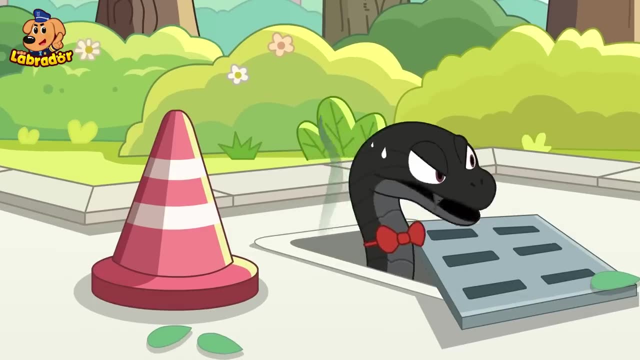 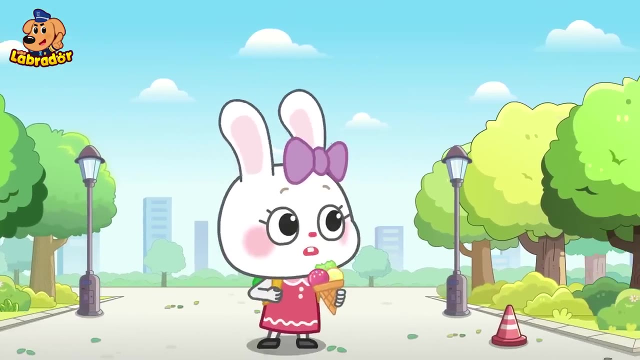 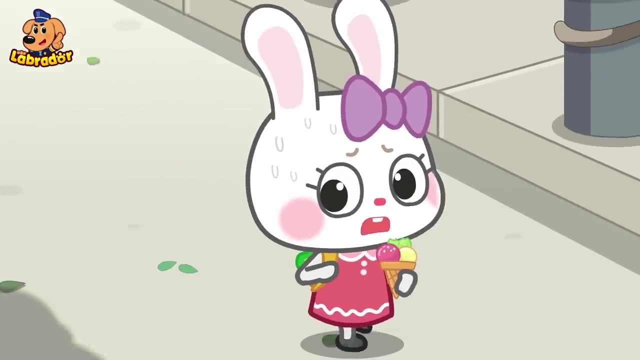 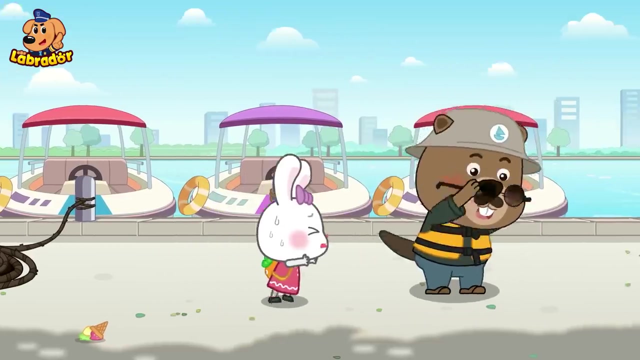 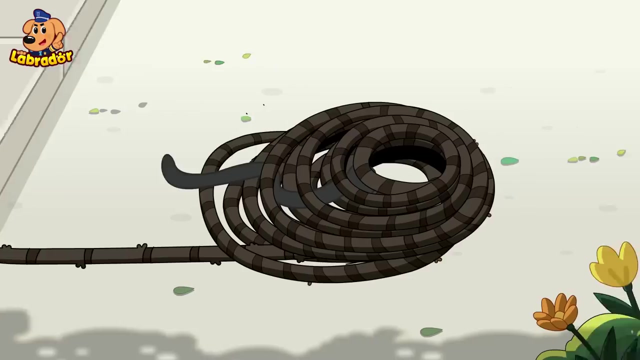 Bye. The kid is alone. It's my chance to take her. So, yummy, What's that sound? Who is it? Mr Beaver, there's something strange in that pile of ropes. Let me take a look, Kid, this is just a normal rope. Look. 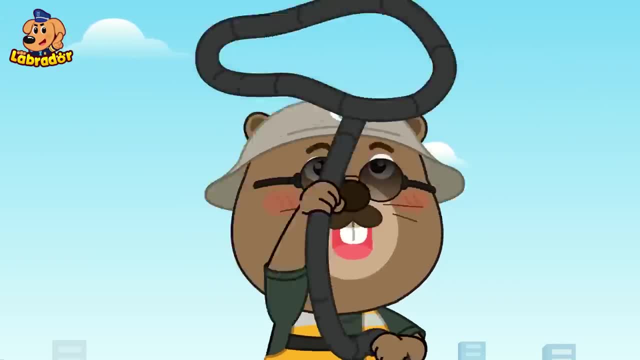 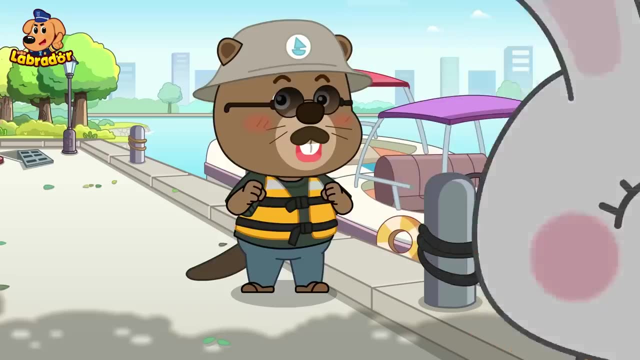 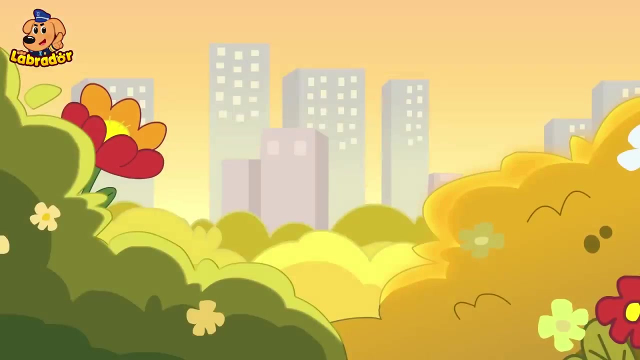 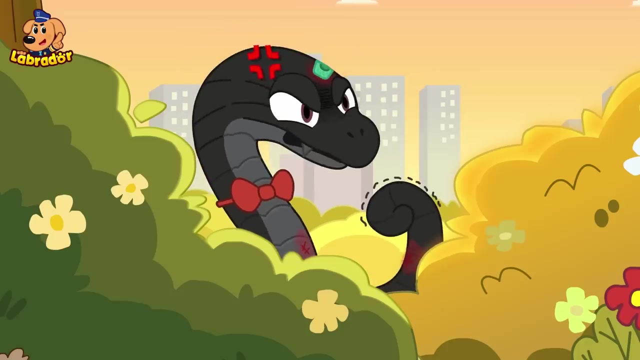 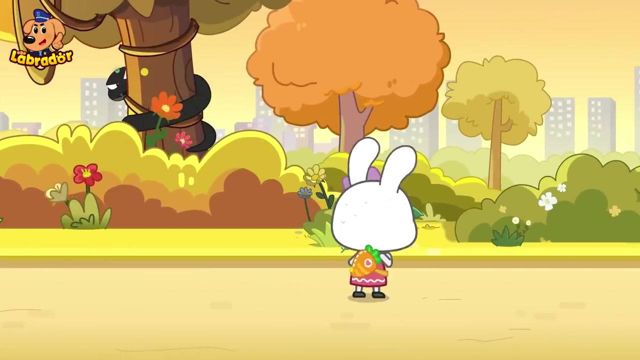 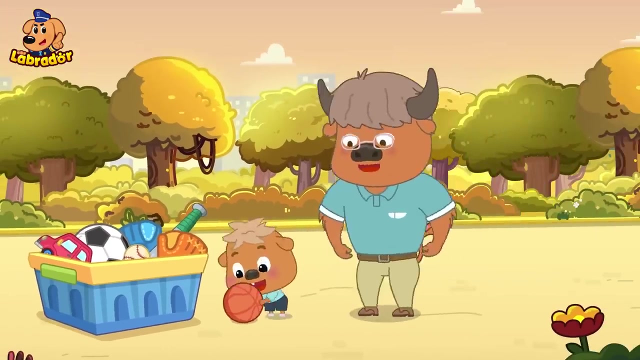 Oh, thank you, sir. You're welcome. Where did the rope go? I'm gonna catch you. Oh The strange, Oh the sound. again, Who's following me? Daddy, can you teach me to jump rope? Of course. 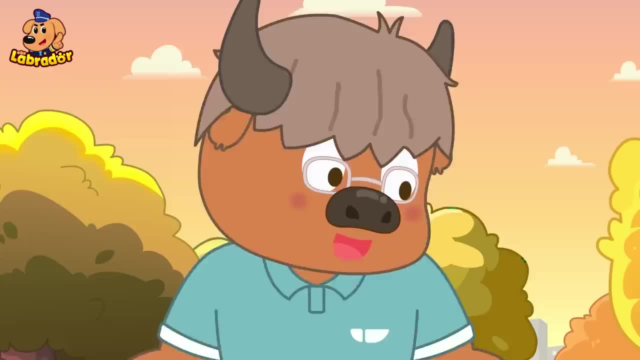 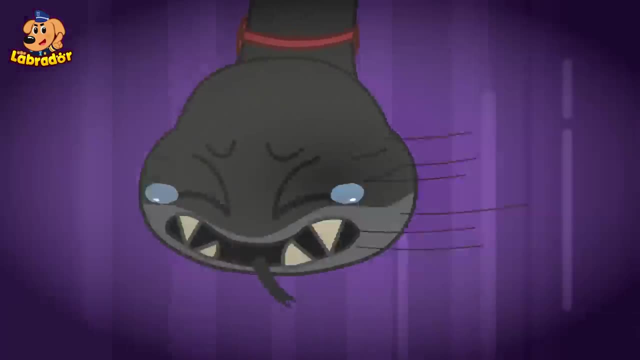 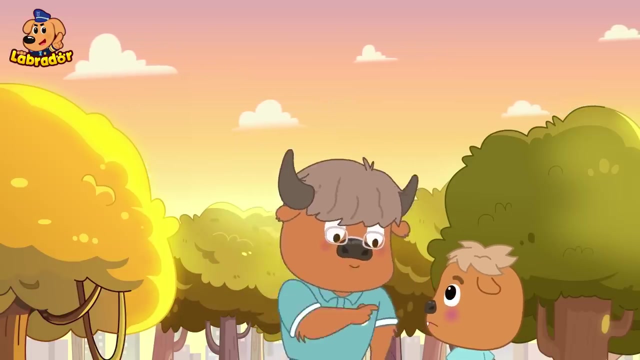 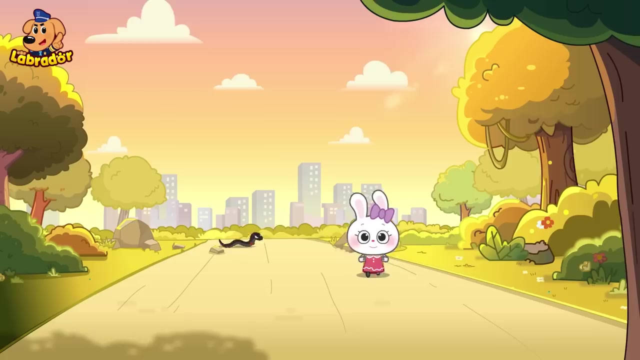 Again, Daddy, Awesome. Oh, Oh, Oh, Oh, Oh, Oops, The rope is too slow, Too slippery. Haha, Son, let's just go play soccer. Yeah, Oh, oh, oh, oh, Huh, Huh. 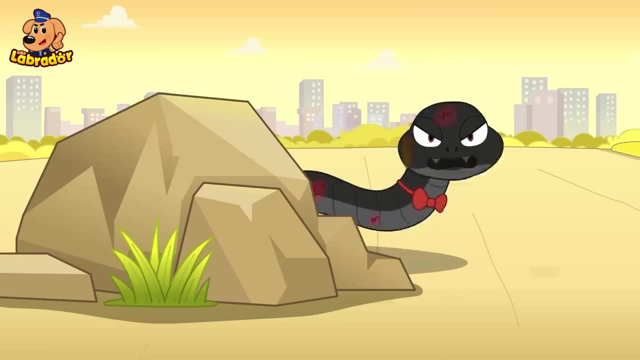 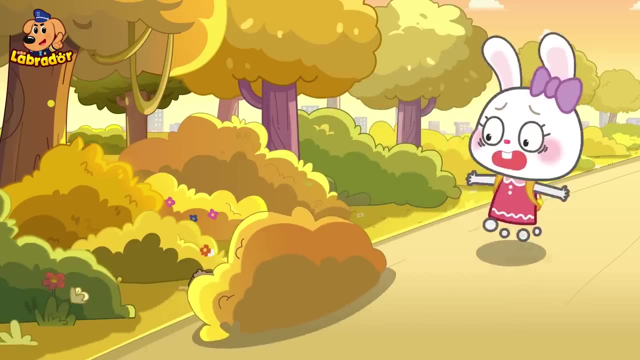 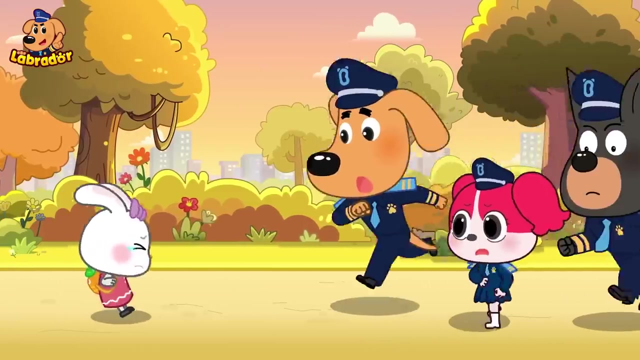 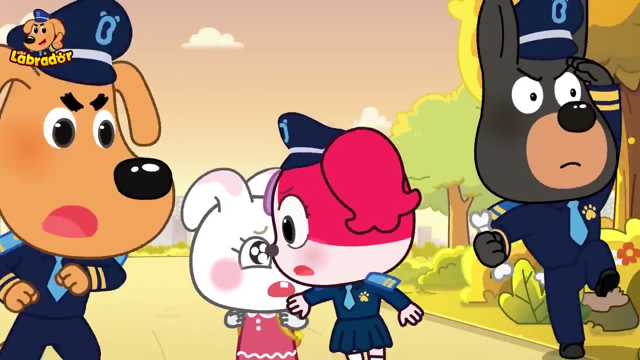 Huh Ha, I'm gonna catch you this time. Hmm, Huh, Aaaaah. Sheriff Labrador, Stop The police. Someone's following me, What? Don't be afraid, little rabbit, We will keep you safe. 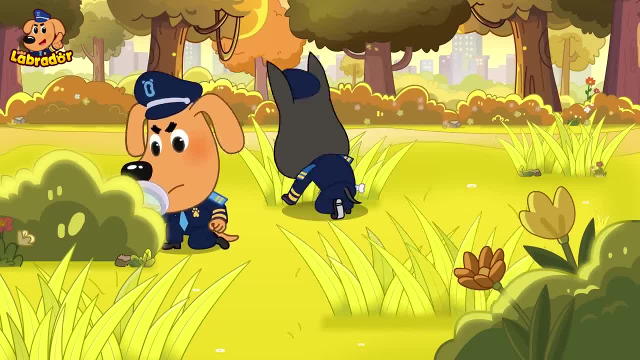 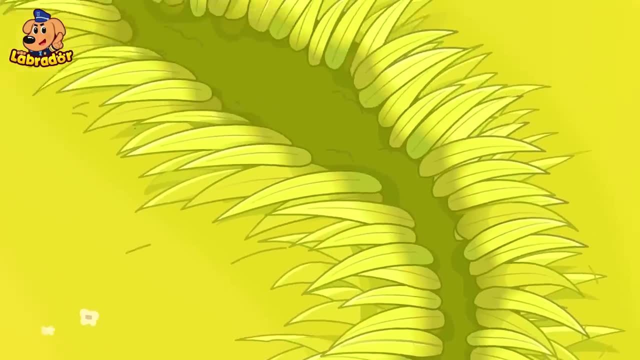 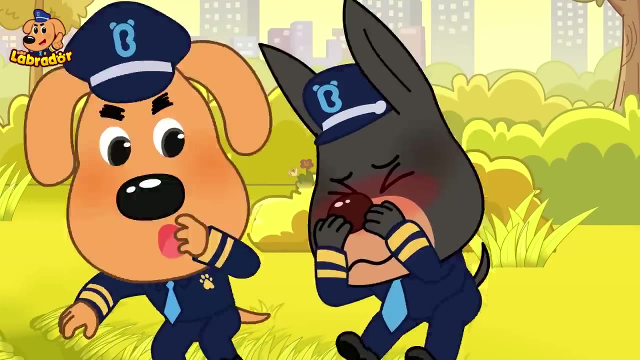 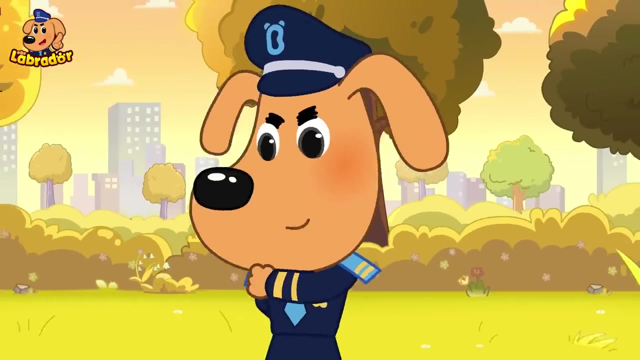 Let's go check it out. There's no one here. This is the trail of a snake. What's this? This is Black Mamba's scale. It's Black Mamba who's following little rabbit. It's him again This time. he won't get away. 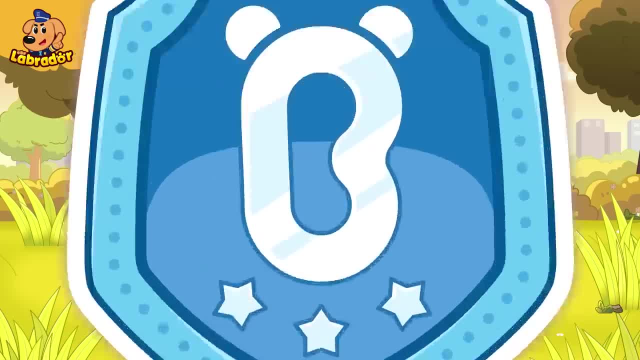 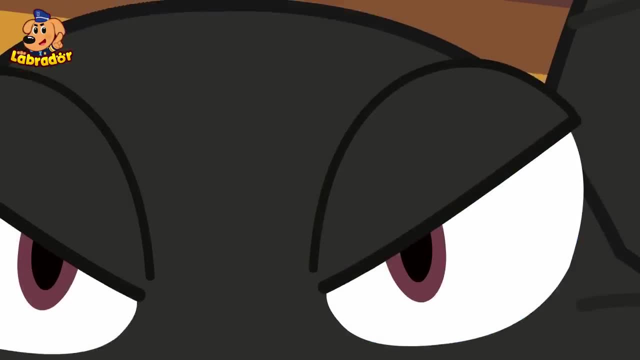 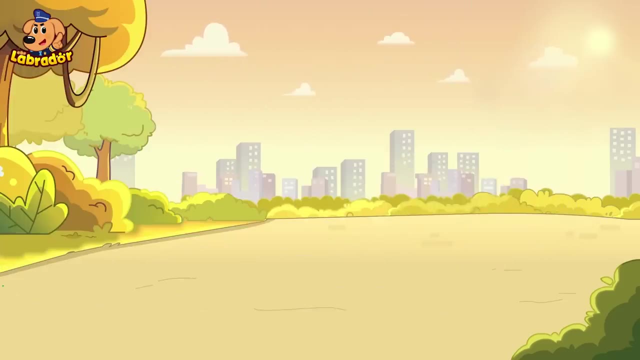 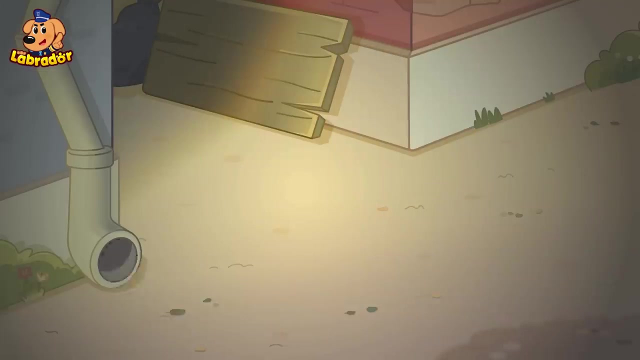 That's it, Little rabbit. we looked around. No one's following you, Don't worry, just go home. The police couldn't find me. I'm going to catch you, kid. This is a faster way home. A perfect place to catch the kid. 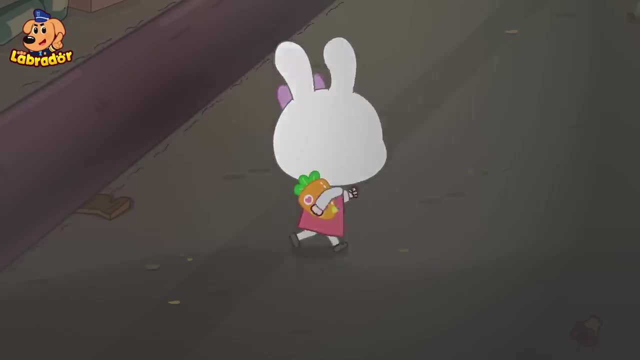 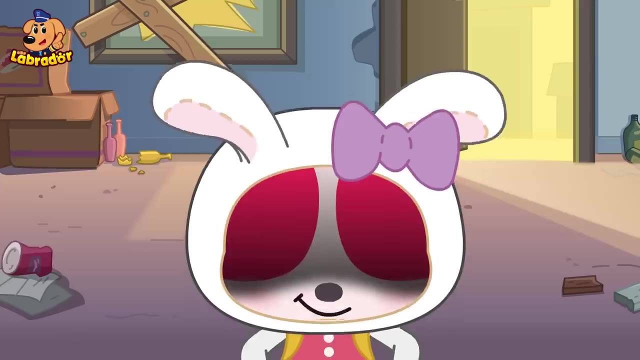 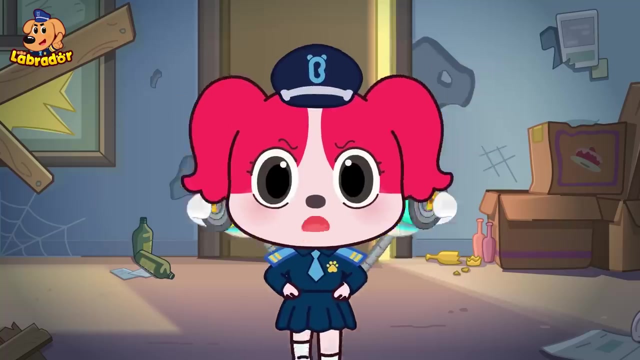 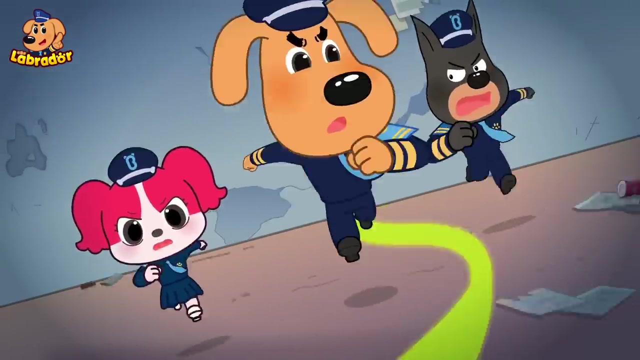 Don't run, little rabbit. You can't get away. I wasn't planning on getting away The police. We've already seen through your tricks. This is called blurring the snake. You've got neon spray paint on you. You can't run away. 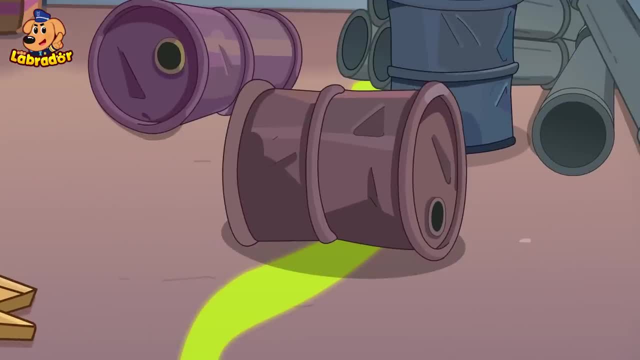 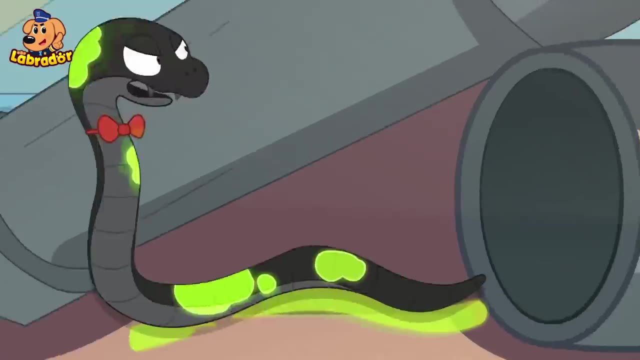 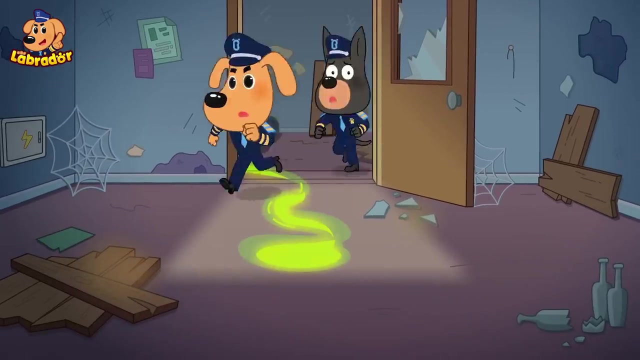 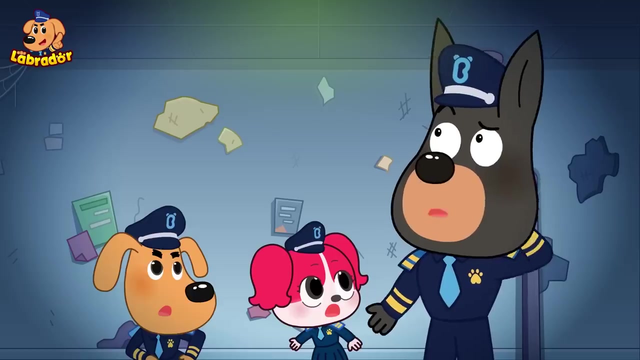 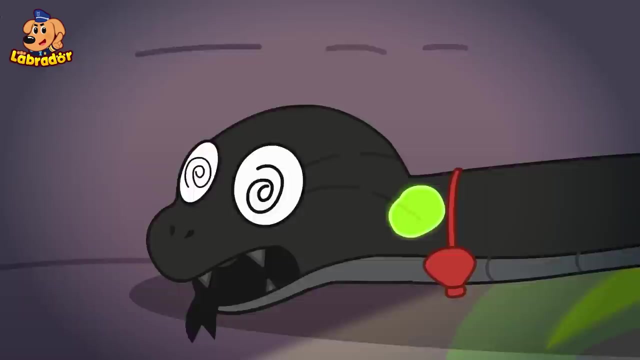 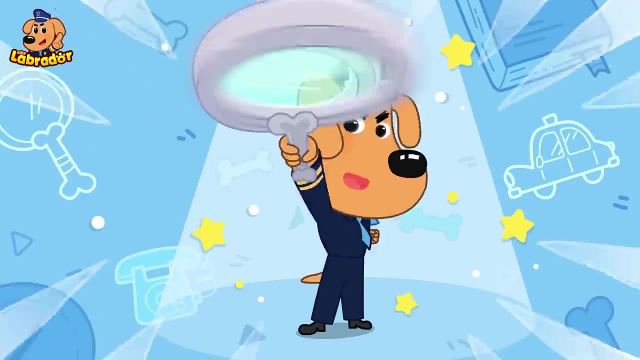 Chase him. There you are. The paint stopped here. Why is there a light here? No, That's Black Mamba. They found me. Nobody can run away from me, Sheriff. We've found thecau and thecau.